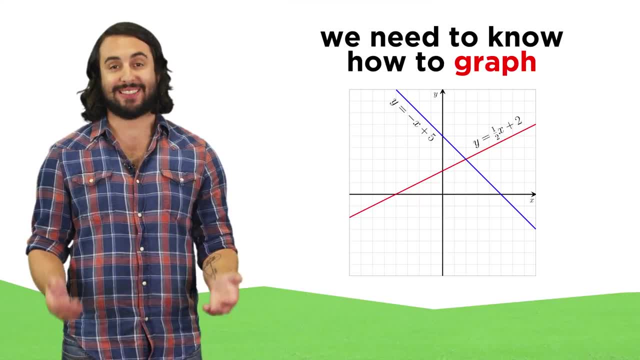 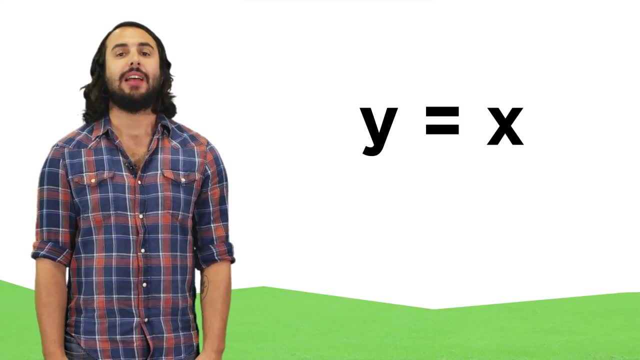 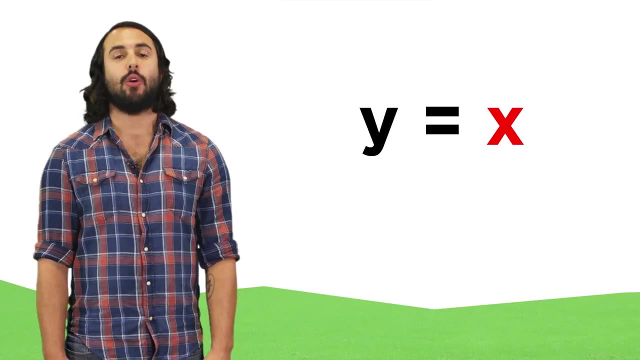 as well, because graphs are visual representations of equations that help us comprehend the relationship between two variables. Let's take an incredibly simple equation: Y equals X. This says that whatever X is equal to Y is equal to that too. so if we make a chart of X values and their corresponding 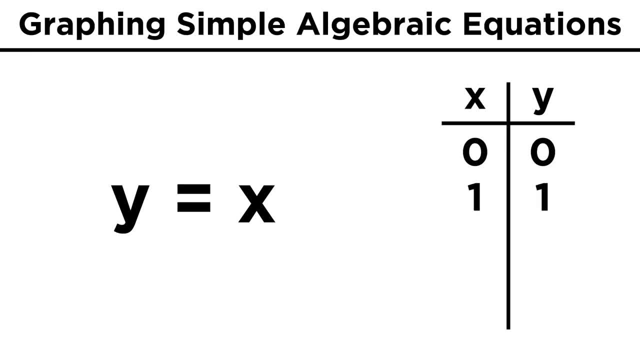 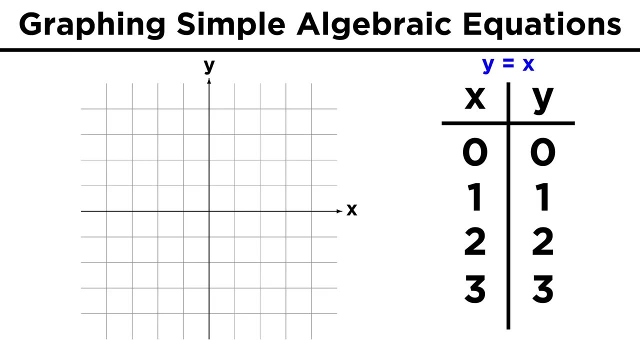 Y values, we get zero and zero. one and one, two and two. This could continue to infinity, in either direction. Is there some way we can draw a picture that demonstrates this relationship? Why don't we draw a grid? On this grid, which we call the coordinate plane, we can create two axes: the X axis. 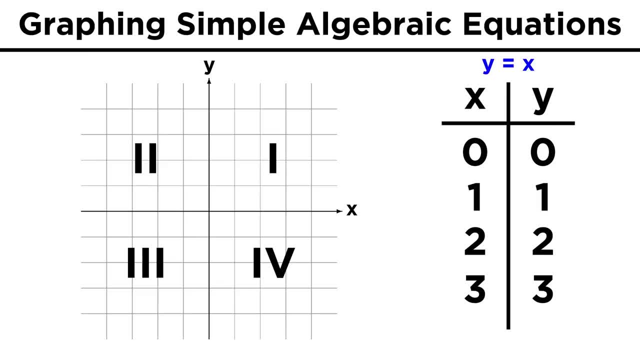 and the Y axis, which split the plane up into four quadrants. Those are quadrants one, two, three and four, represented by Roman numerals. By convention, the X axis is the square root of the square root of the square root of the. 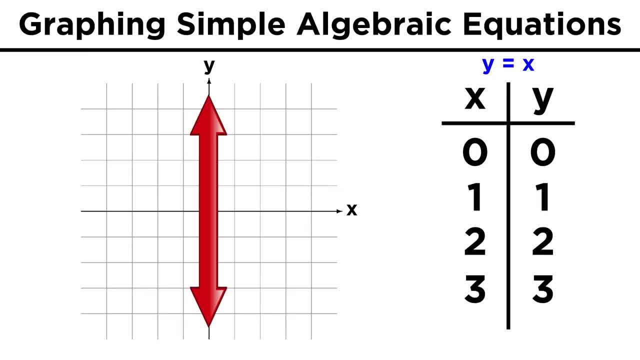 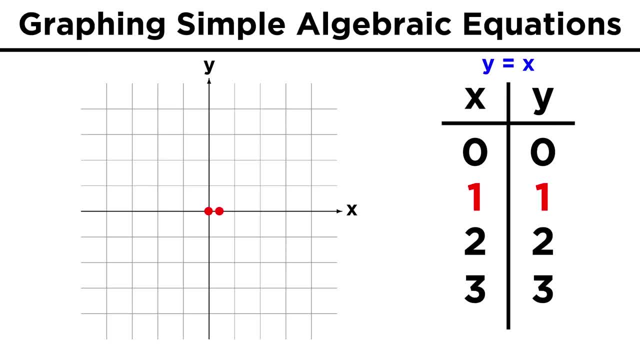 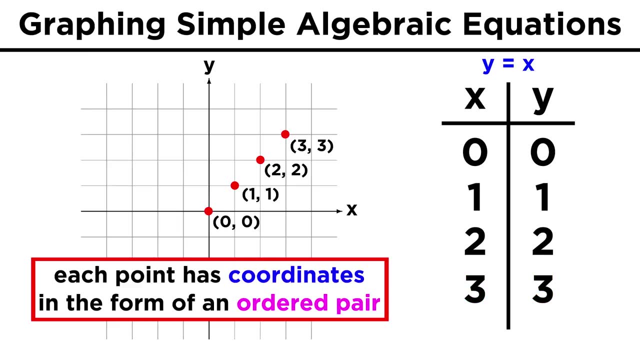 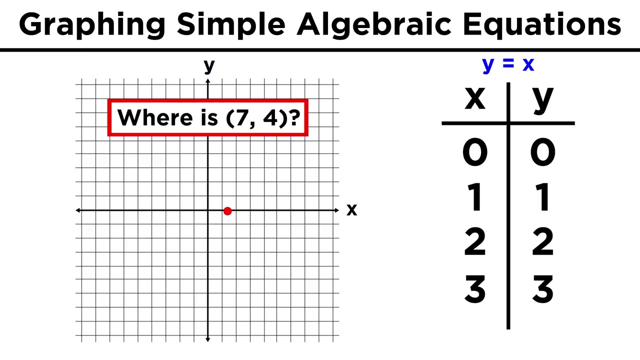 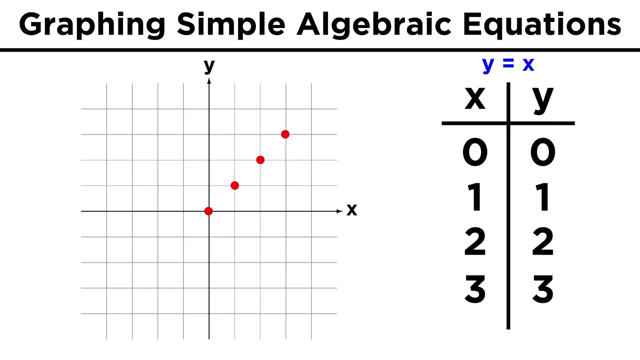 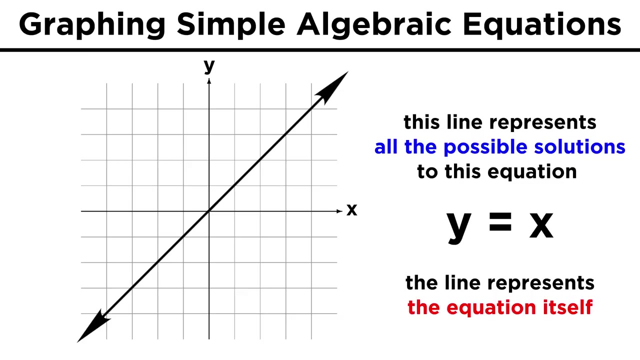 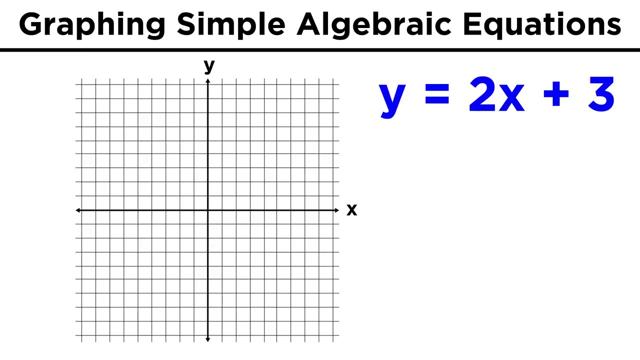 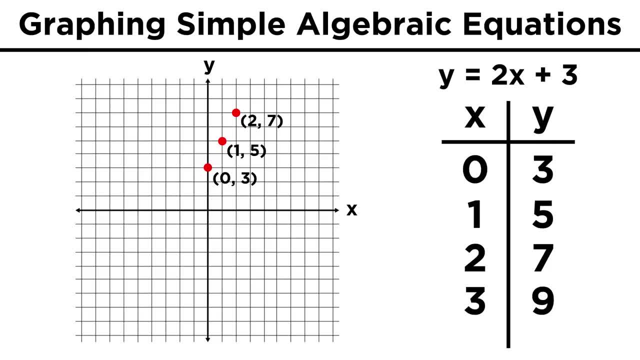 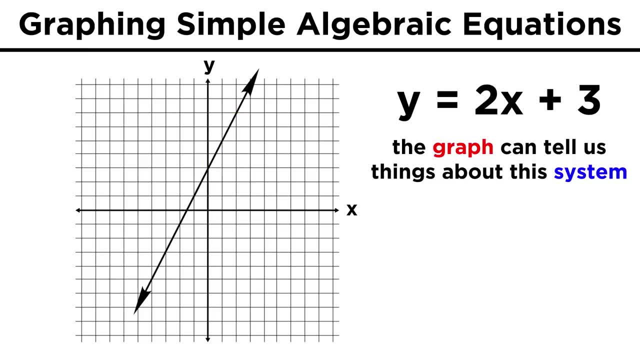 is listed. remember, it's the X value first, then the Y value. we connect the dots and there is our line now. the interesting thing about graphing these equations is that we can use the graph to make inferences about the system equation instead of having to do any math. 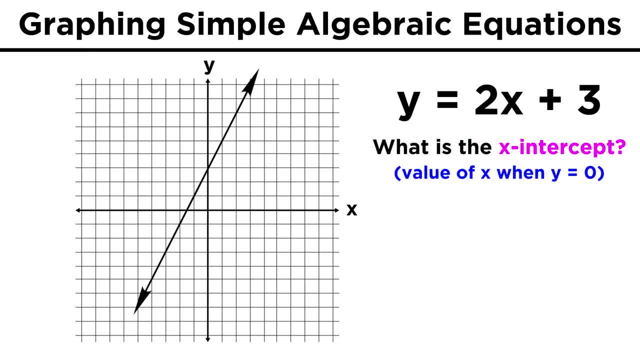 Say, we take this same equation and we want to know the value of X when Y equals zero. We can trace along this line until it crosses the X axis, and right where it touches the X axis is where Y must equal zero. At that point the X value is right in between negative one and negative two, so it must. 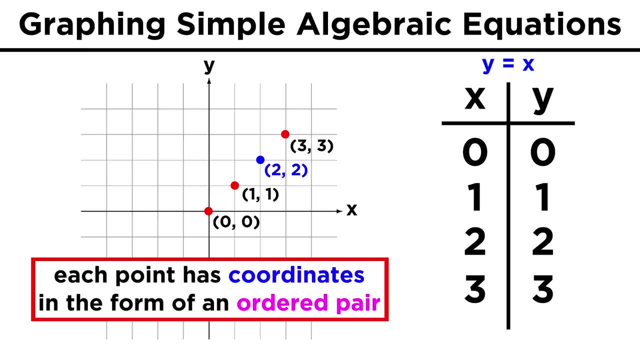 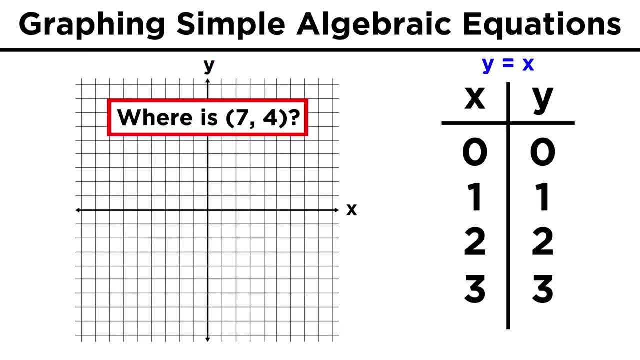 That means two comma two will correspond with this point, and we always list the X value first, followed by the Y value. If we want to find seven comma four, we start at the origin and go seven to the right, then up four. 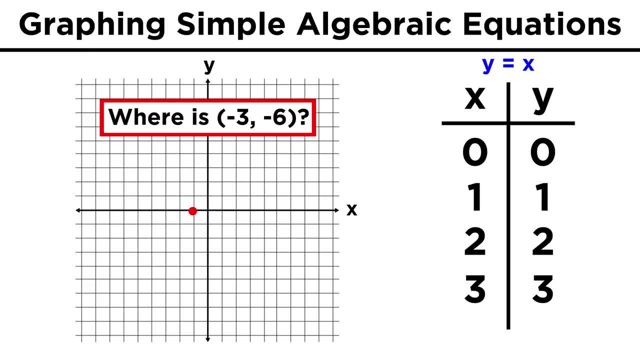 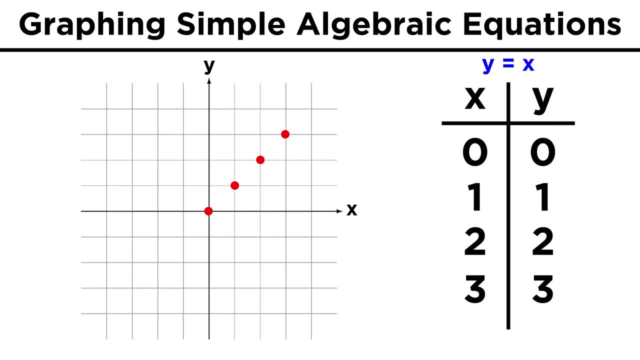 If we want to find negative three comma negative six, we start at the origin and go three to the left and six down, as left and down are the negative directions for X and Y respectively. Now, with all these dots pertaining to our original dataset, we may as well connect them, because it's not just 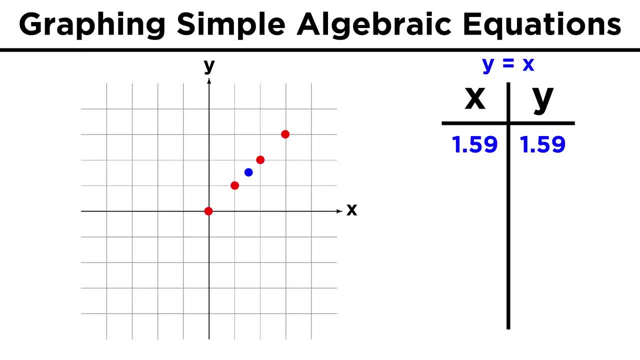 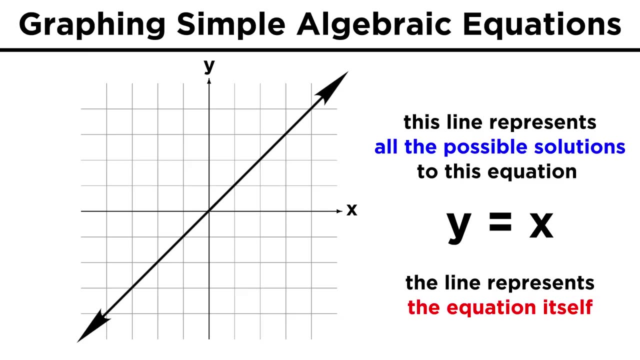 integers that satisfy this relationship. If X is one point five nine, so is Y. If X is two hundred sixty seven, one hundred twenty-fifths, so is Y. So this line contains all the possible real numbers that satisfy this equation. In this way, the line represents the equation Y equals X. 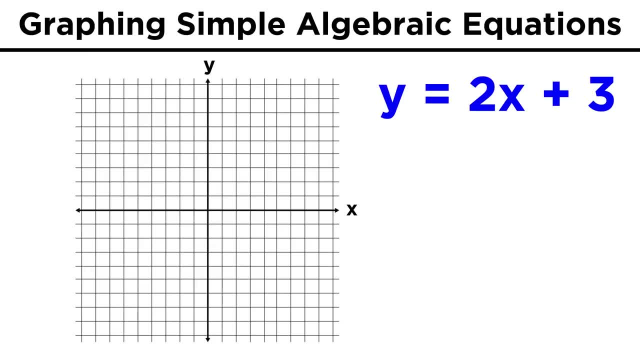 Let's try another: Y equals two X plus three. Again, we can make a table where we choose any numbers we like for the independent variable X and see what values we get for the dependent variable Y, which depends on the value of. 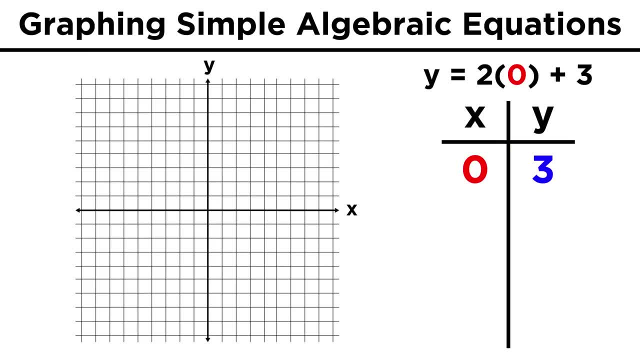 X for its own value. When X is zero, Y is three. If X is one, Y is five. If X is two, Y is seven. So we can see the relationship between X and Y begin to emerge, even just by looking at. 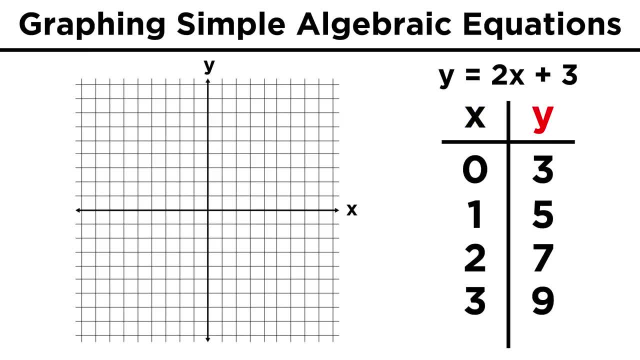 the numbers. Every time X grows by one, Y grows by two Because of this two in the equation, But this relationship is understood more effectively if we draw the graph. Here are the first three points we mentioned, with their ordered pairs listed: 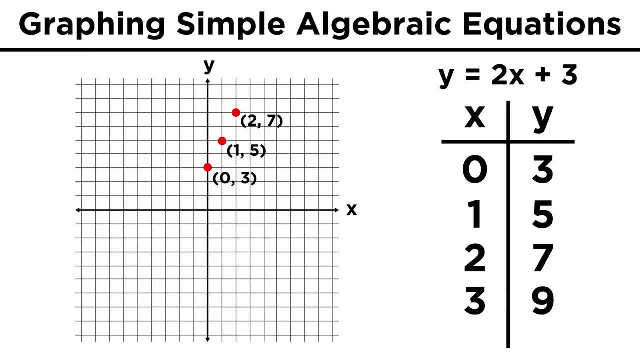 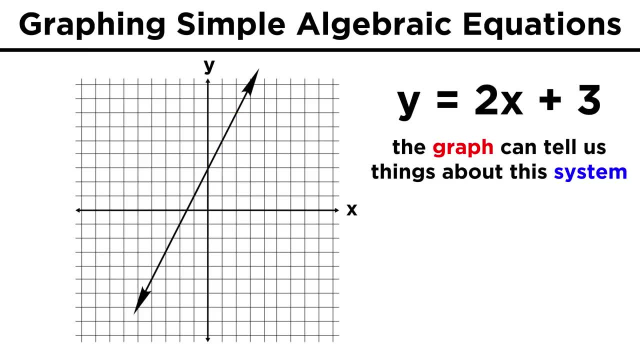 Remember, it's the X value first, then the Y value. We connect the dots and there is our line. Now, the interesting thing about graphing these equations is that we can use the graph to make inferences about the system instead of having to do anything else. 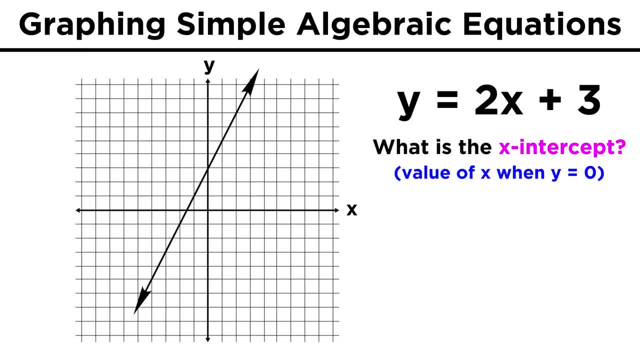 We can use the graph to make inferences about the system instead of having to do anything else. We don't have to do any math. Say, we take this same equation and we want to know the value of X when Y equals zero. 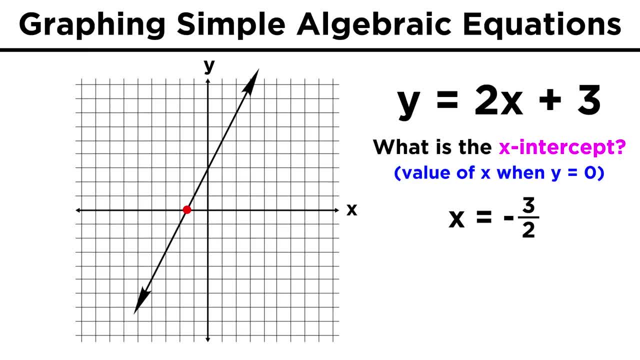 be negative three halves. Of course we can very easily do the algebra to verify this Plug in zero for Y, subtract three, divide by two, and we quickly get the solution that way. but as equations get more complex it won't be possible to do such quick math. 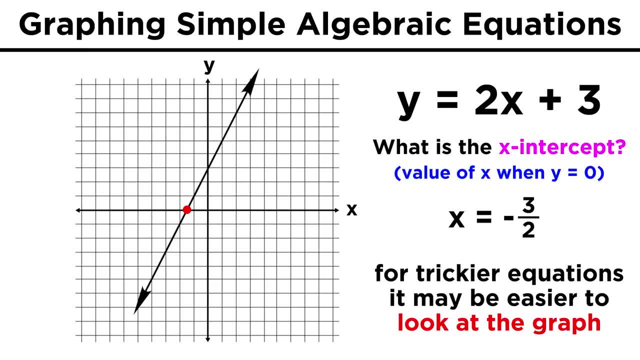 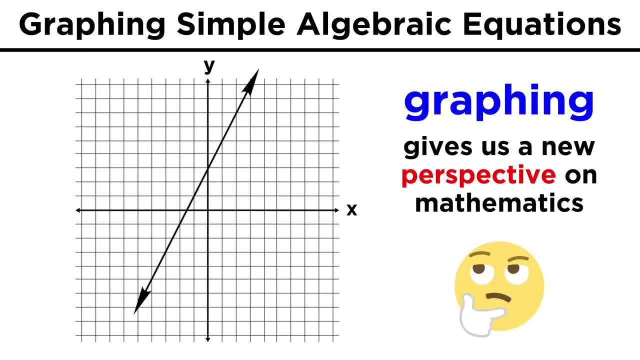 and therefore information present on a graph that we can see visually will become more and more valuable in trying to describe algebraic systems. Also, graphing equations gives us a new and better understanding of algebraic systems. We can view Y equals two, X plus three as simply an equation, or we can view it as the representation. 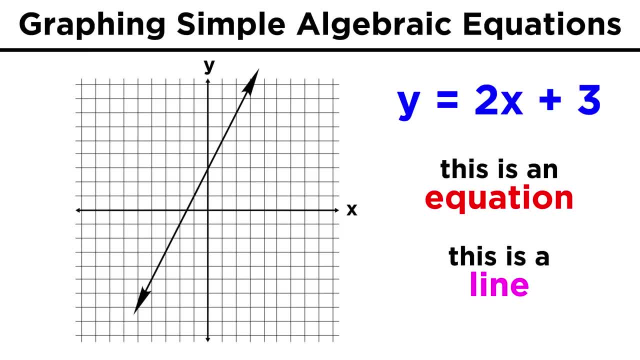 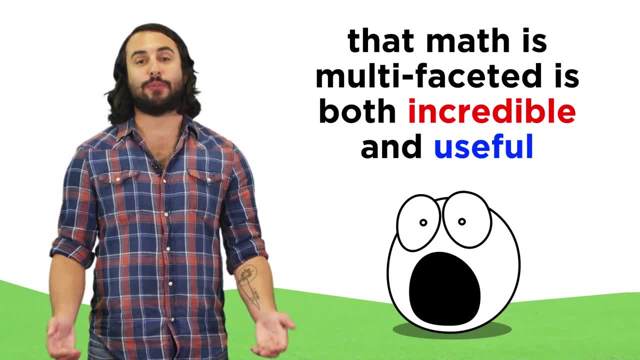 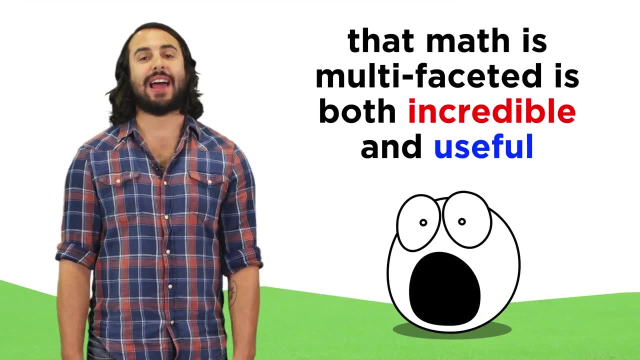 of a line, a genuine geometric object determined by all the points in the X-Y plane that satisfy this relationship. The fact that there are many different perspectives in math is not only incredible but also useful, as a variety of approaches will better allow us to solve a variety of problems. 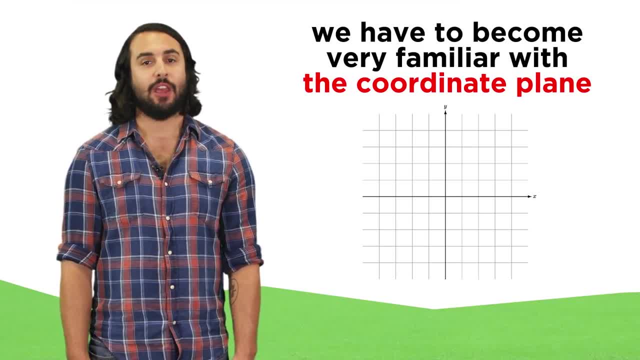 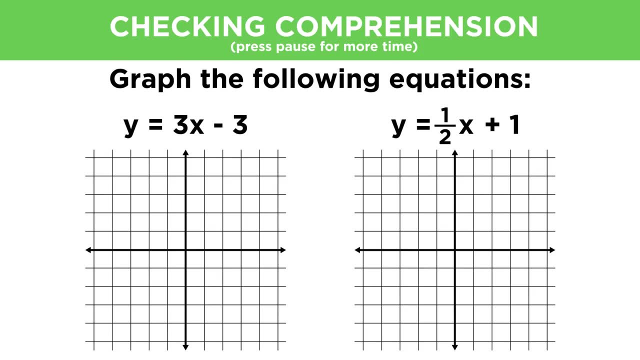 We will be graphing quite a bit throughout our study of math, which means we'd better understand the coordinate plane. so let's check comprehension. Thanks for watching, guys. Subscribe to my channel for more tutorials. support me on patreon so I can keep making. 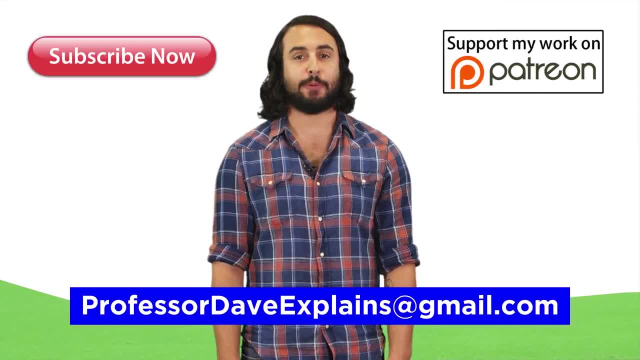 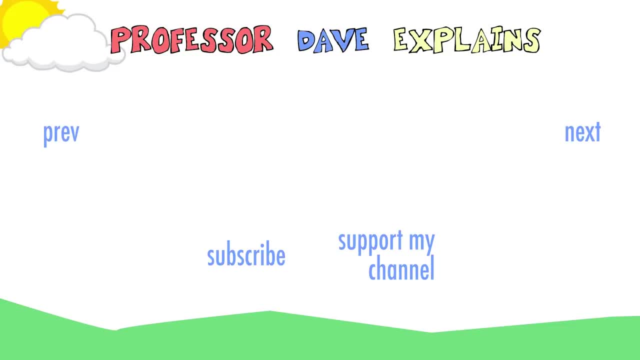 content and, as always, feel free to email me professordaveexplains at gmail dot com. I'll see you next time.